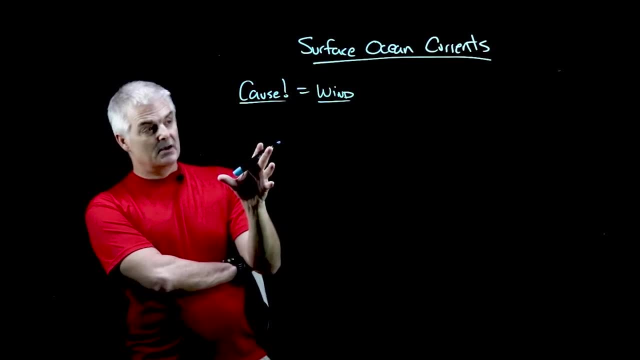 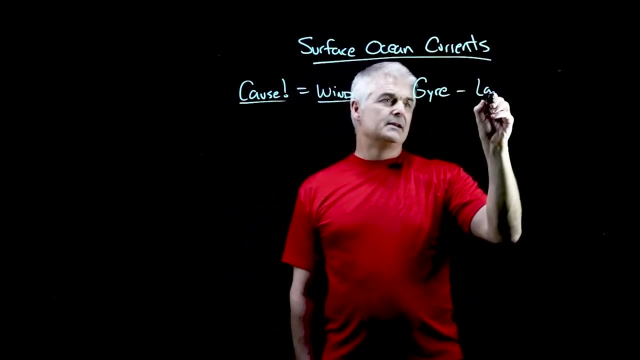 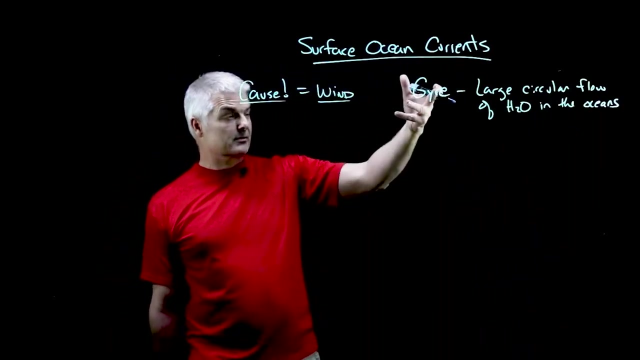 follows the patterns of the ocean currents. But let's also define one more term. It's this one: It's a gyri. And a gyri is a: It's a large circular flow of water in the ocean. Well, the gyri is like Greek or Latin, or 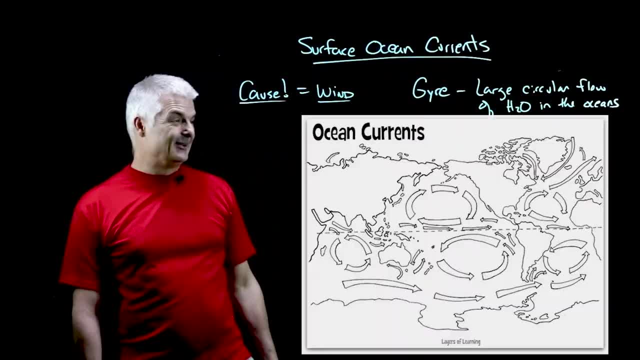 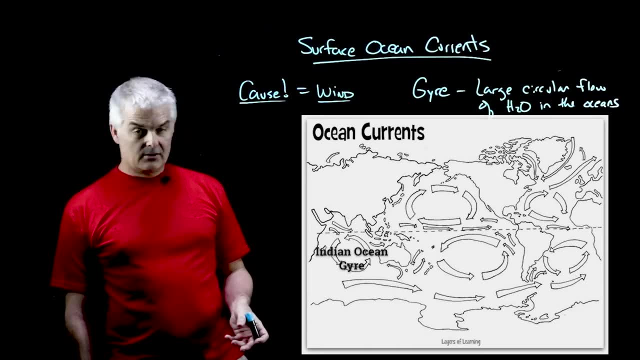 Roman or something Like Latin's Roman, I guess, Over a circle. So take a look at the map and let's talk about the big five. There's five gyris. The first one is the Indian Ocean Gyri. 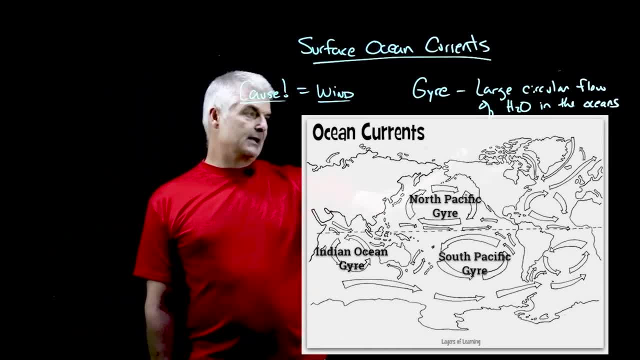 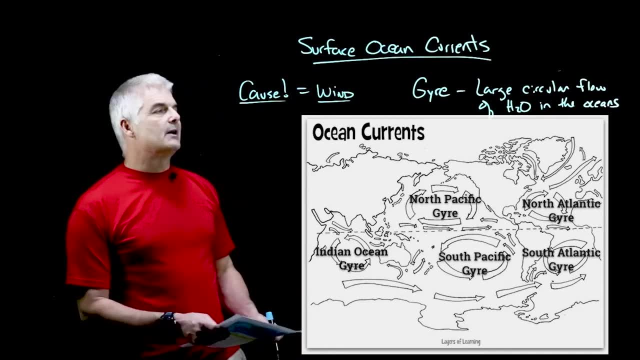 And then we've got the North Pacific and the South Pacific, And then we've got the North Atlantic and the South Atlantic. Make sure you label that in your notes, But let's also do some other additional labeling. Now. we're going to use this graph, though, to help label the rest. 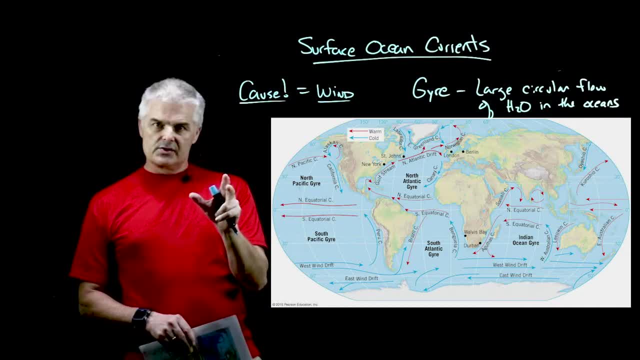 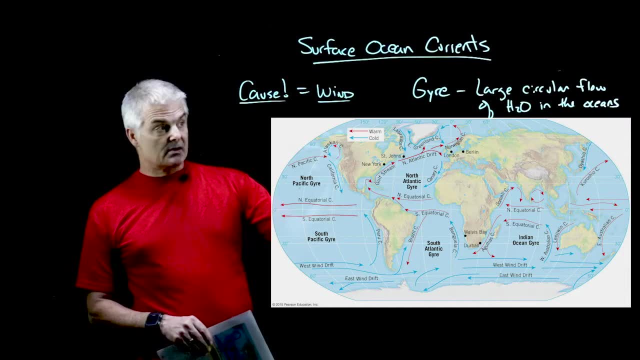 of our graphs. It's a little more colorful one And it's important to note the blue verses, the red. The blue means that it's cold, the red means that's warm, And you'll notice the pattern is the red ones tend to come from the equator, the blue ones come from the poles. Cold versus hot water. 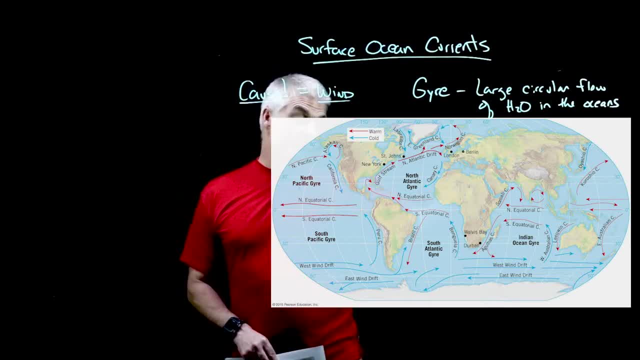 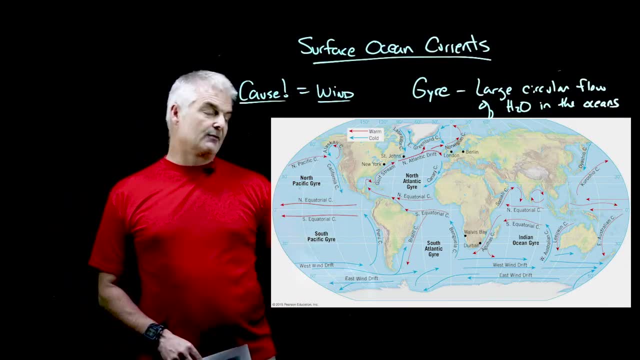 So let's label a couple of critical ones. This one, across on the east coast of the United States is the Gulf Stream. It flows up from the equator, And on the other side of the United States you've got the California Current. 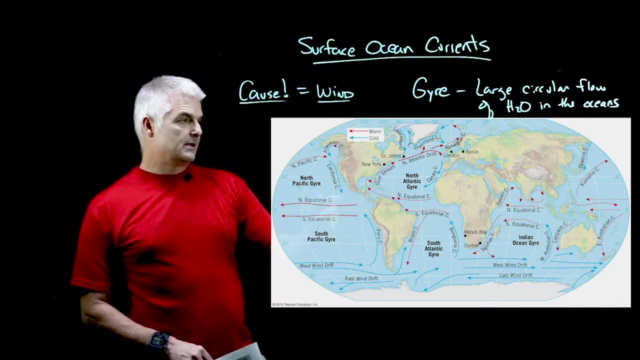 Do you see that? And the California Current is cold. That's something. I don't know if you've had a chance to be on both coasts, But the water off the coast of the Atlantic Ocean on the United States tends to be warm water. 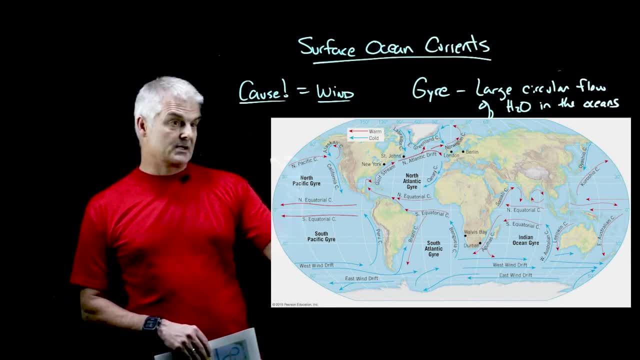 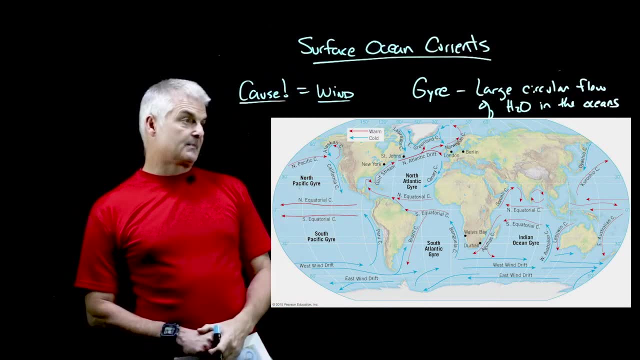 And in California Coast it tends to be much colder because it's coming the current right on the edge of the Earth. These are part of both the Atlantic and the Pacific Gyrie, But these are important currents. Notice some other currents on there. 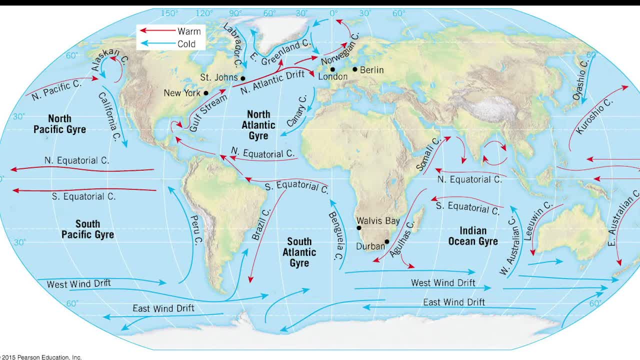 There's an interesting one that I think is really important. It's at the bottom of the graph. right here is we have the west wind drift and the east wind drift. Not all of these are on the map that you're going to be filling out in your notes. 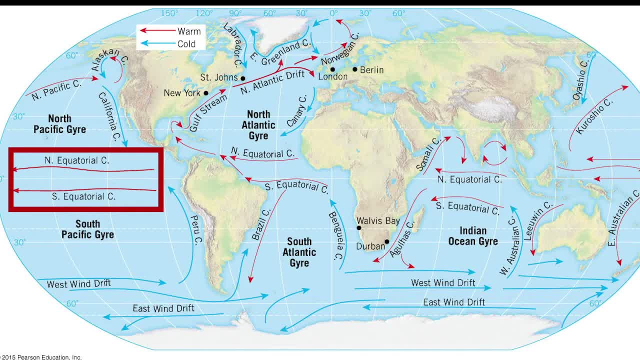 But also that there's the north and the south equatorial currents across the middle, et cetera, et cetera. I think another one that would be interesting to measure is the North Atlantic Drift, That's that one that shoots up to England and stuff. 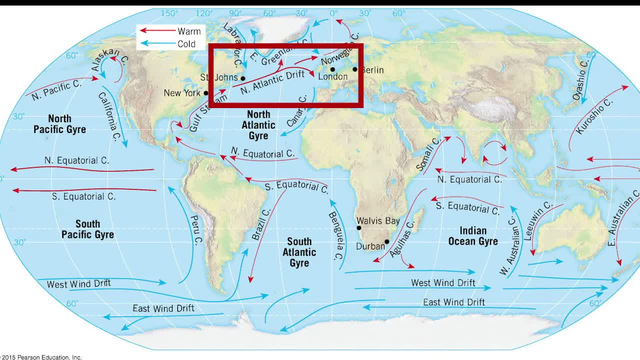 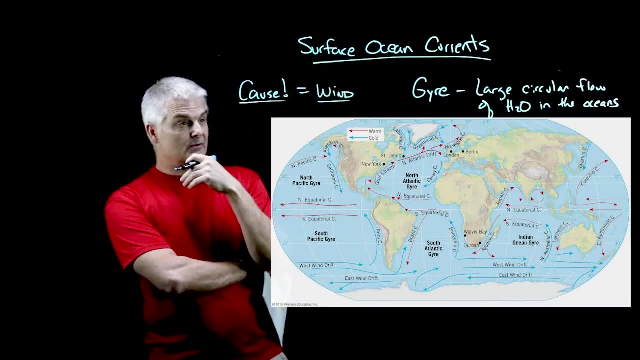 And because of that warm water this actually affects the climate of the world. is that that keeps England and whatnot warmer? Because if you kind of go across to an equal latitude you would find in the United States- actually it would be in Canada. it would be a super cold place.